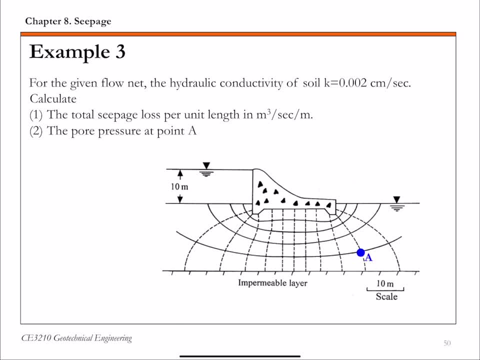 application of flow net to solve seepage problems And for this given flow net. first, the information we can get from this graph includes the upstream water table. This is what we typically call H1.. And then downstream water table. we call H2 here And for this. 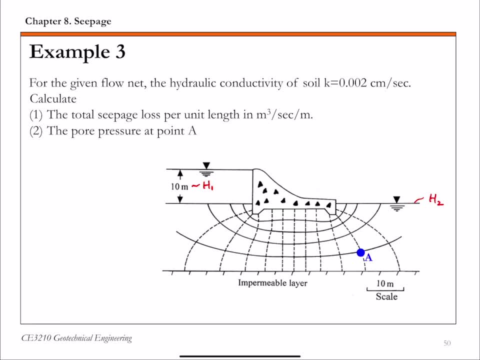 particular setup. the downstream water table is actually at the level of the ground surface. So this is what we're going to do And we're going to put the datum at this downstream water table. So I'm going to put datum here for our calculation. So the total head loss- we call capital H- is H1 minus. 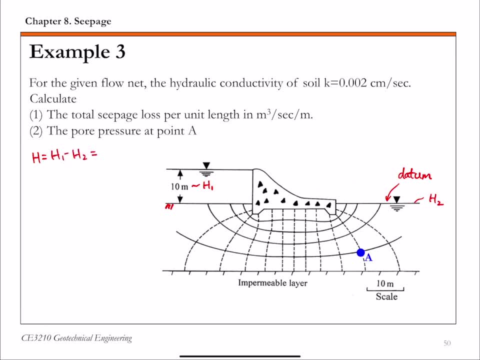 H2 and is basically 10 meters. And also, given this flow net, we can get the number of flow channels we call NF, And for this flow net, we can get the number of flow channels we call NF. And for this. 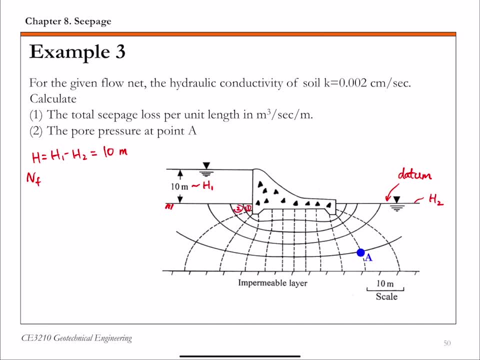 flow net we can get the number of flow channels we call NF, And for this flow net we can get the number of flow channels. so if you say NF, in that if we count it's 1,, 2,, 3,, 4 and 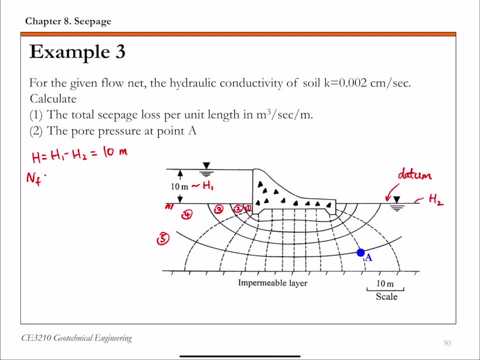 5.. So the number of flow channel NF is 5.. And then the number of equal potential drop or per minimum proper potential drop. So if we start from upstream, so let's use this bracket 1 here and 2.. So if you count 3,, 4,. 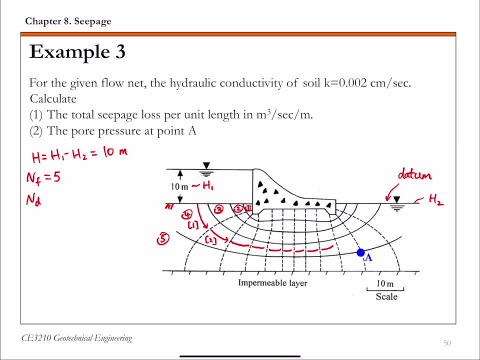 5,, 6 and 7.. Now we're able toçosmer it And then we can look at H1 average potencial six, seven, eight, nine, 10,, 11, and 12.. So there are a total of 12 potential drops. 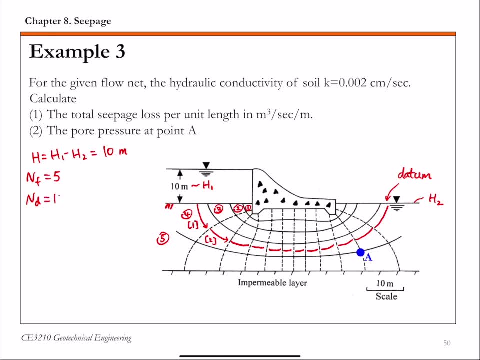 from upstream to downstream. So ND is 12.. And then the potential drops between two adjacent, equal potential lines. So that's basically one delta H, one delta H. So this delta H is capital H. That's a total loss from upstream to downstream. 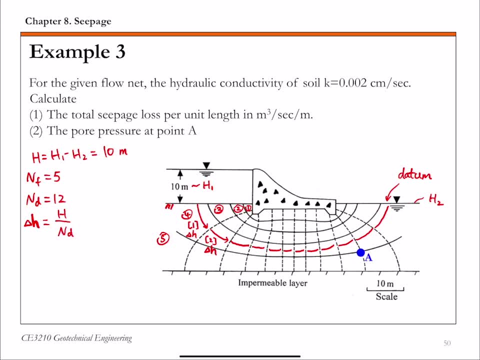 over ND number of potential drops, And this is- let's see plug-in numbers- 10 over 12, 0.833 meter. So that's what we can read directly from the graph and also that potential drop, delta H, we can calculate. 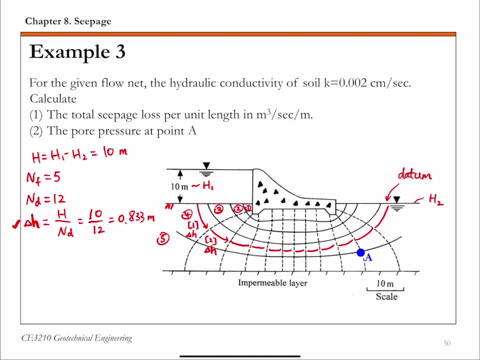 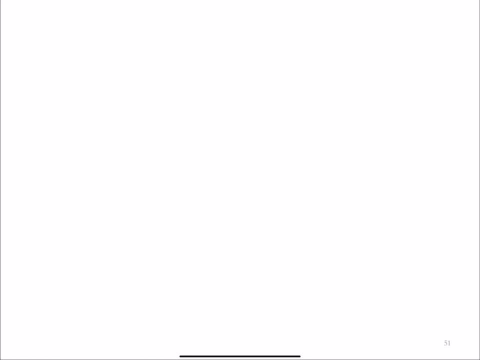 given this flow net, And now let's calculate the total seepage loss per unit length and also per partiality. Let me open up blank page here. So first for part one, we're going to calculate this small Q here. So for this flow net, 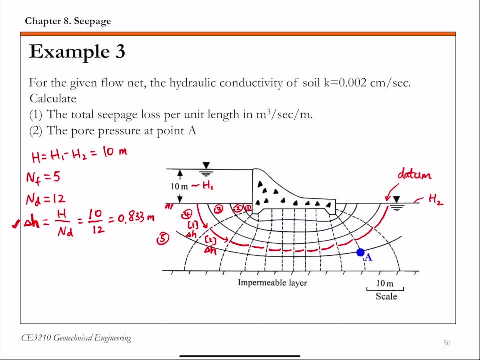 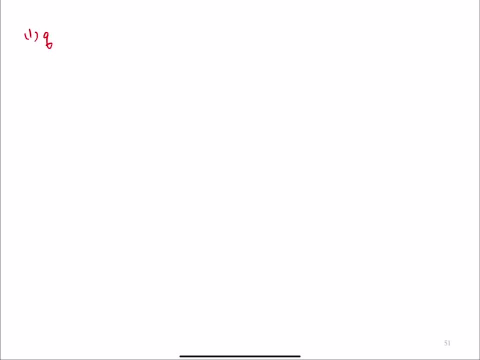 so all the flow net elements have aspect ratio or has a ratio of length to width of one. So they're all approximate square elements. So Q- we can use this equation here- K times H over, ND times NF. so that's for flow net with. 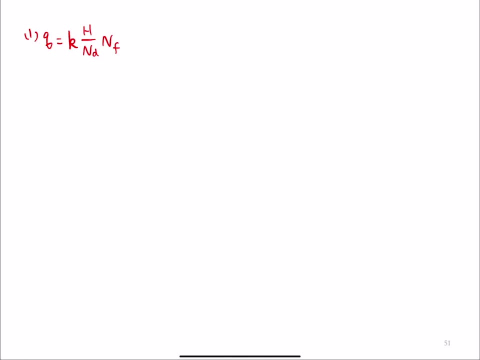 square elements. so unless otherwise stated in the problem, we can assume this L over B value is 1, so we can use this equation for square elements. so this is 0.002 and this is centimeter per second. so I'm going to convert that to meter. 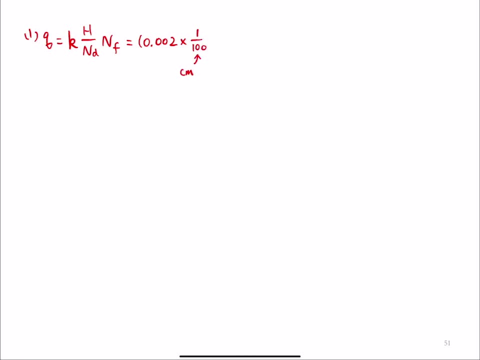 per second. so this is from centimeter to meter conversion factor. then H is 10, ND the quantity is 12 and NF is 5. so if you plug in numbers you get 8.33 times 10 to negative 5 meter cubed per second per unit length meter and then you can convert this to: 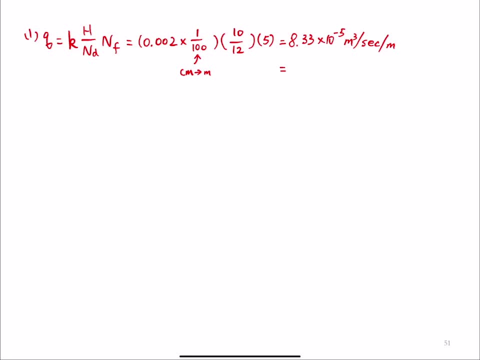 meter cubed per day per meter. so that's 7.2 meter cubed per day per meter. so that's part 1, the seepage quantity per unit length. and then for part B, part 2, we want to know the pore pressure at A. 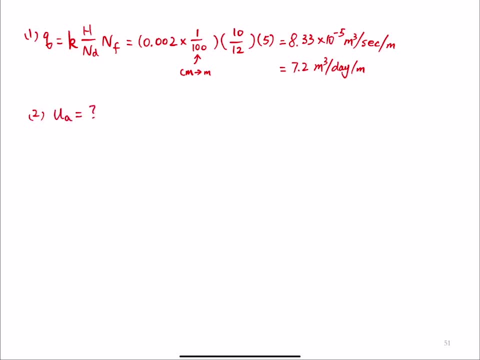 so we want to know the pore pressure at A. so we want to know the pore pressure at A, U or capital a. so, just as what we did for in here, example 2- and for to determine the pore pressure, the watercolor at A, we need to. 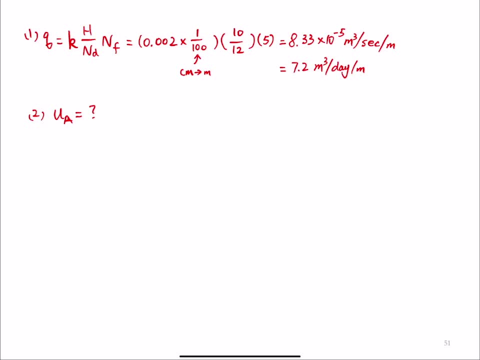 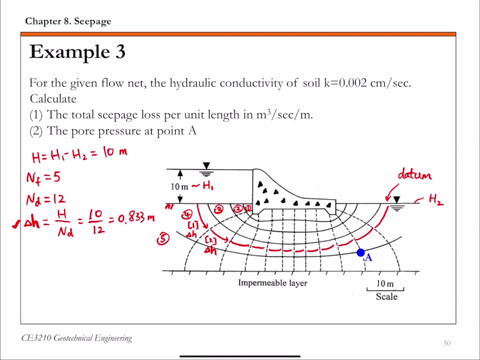 just as what we did for in example 2, and therefore to determine the pore pressure, water pressure at A, we need to know the total head at 8. so let's look at this graph here. so when water travels, the total head at 8. so let's look at this graph here. so when water travels. 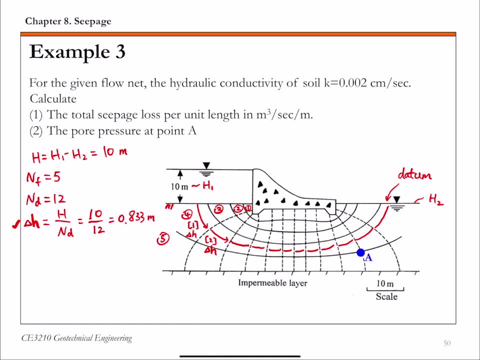 from upstream to point A. so let's count how many potential jobs water experiences. so that's, that's the result in the graph. so the total air flow is Sudor planning. we're going to take water 3480 and we need to exactement provide you bringing in water Teraz. 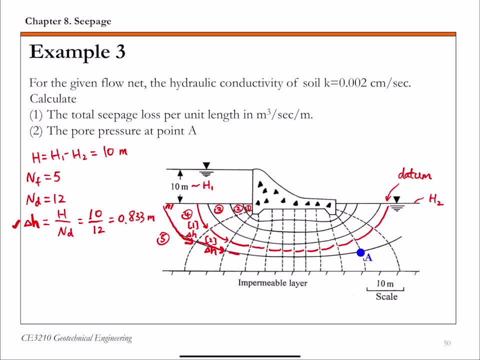 1,, 2,, 3,, 4,, 5,, 6,, 7,, 8,, 9, and 10.. So in total, Walter experiences 10 potential drops from upstream to point A. So remember, each time you cross a equipotential line the total heavy is lost by delta H. 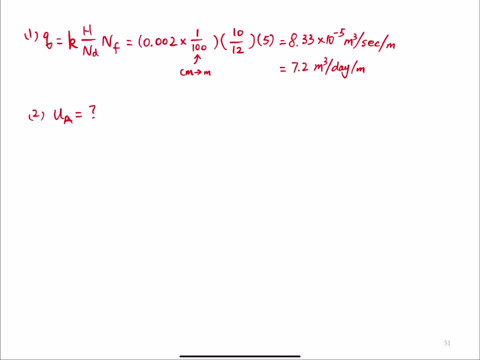 So you have one potential drop, But then for point A, so at point A. so Walter experiences 10 equipotential drops, 10 delta H, So that's counted from upstream. So then the total head at A, we call H A. 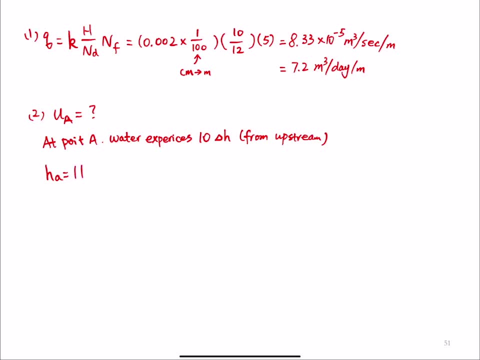 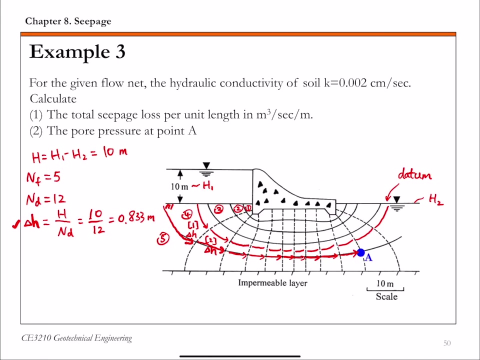 is the initial head in the water at upstream we call H1, minus the head loss, So that's 10 delta H, And the initial head at upstream is 10 meters above the datum, the reference datum at the ground surface, minus 10 times delta H, which we calculated is 0.833 meters. 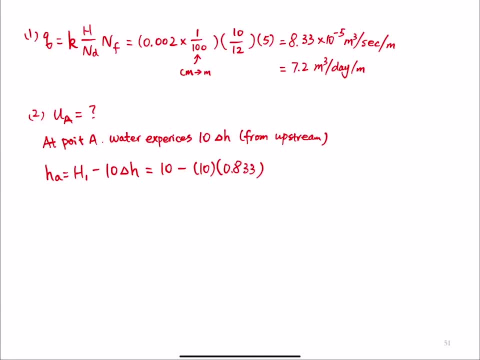 0.833.. And then the total head at A is 1.67 meters. This is above or say with respect to ground surface. So ground surface is our datum, And then the elevation head is Z A And Z A is something again you read directly from the graph.